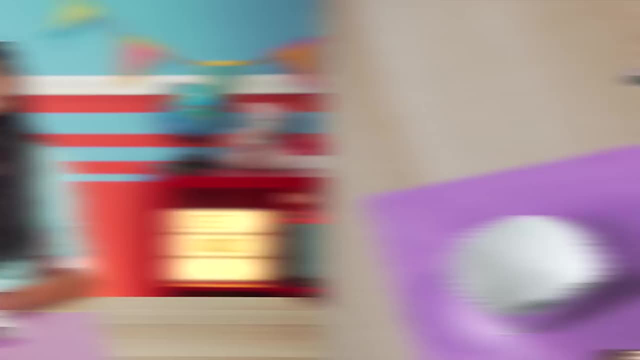 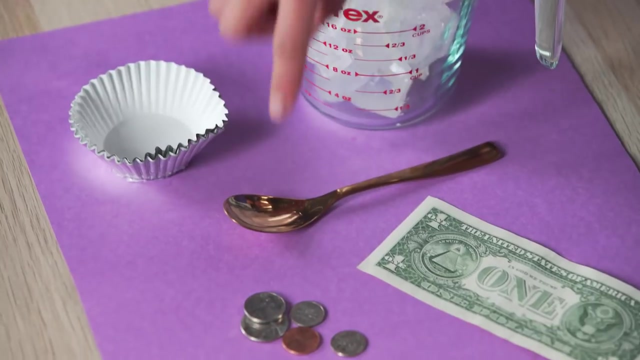 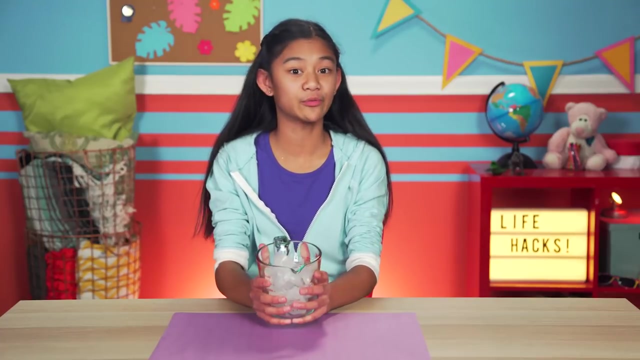 It's my clean, cold cash soap. For this hack you'll need clear glycerin soap, a measuring cup, foil, cupcake liners, a spoon money in both dollars and coins, and plastic wrap. First step: ask an adult to help you microwave your chopped up glycerin soap for about a minute and a half. 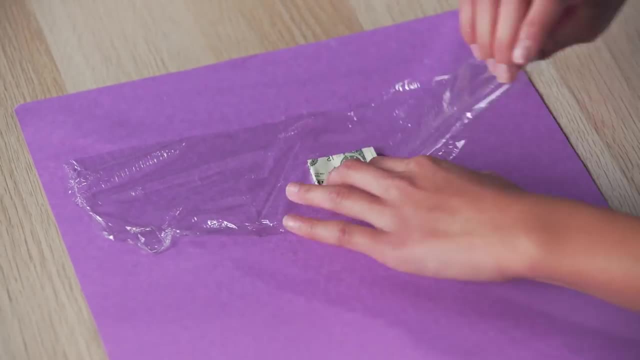 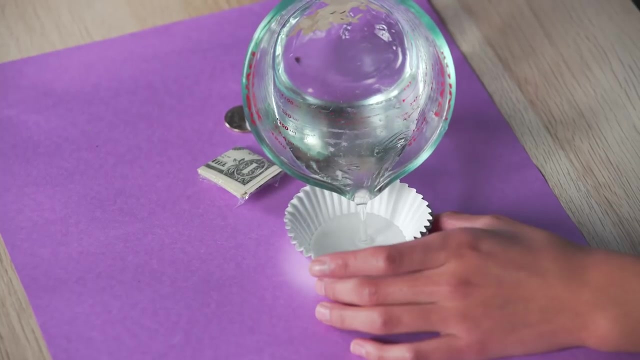 If you're using real dollar bills, make sure to fold them up and to protect them with your plastic wrap There. protect it. Pour a little of the soap inside your cupcake wrapper. Be careful when you're working with hot soap. Add the bills or coins any way you like. 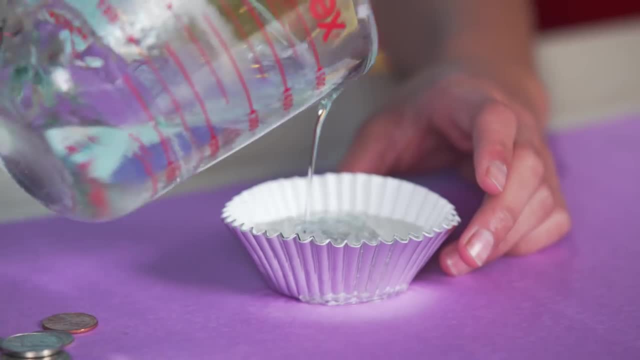 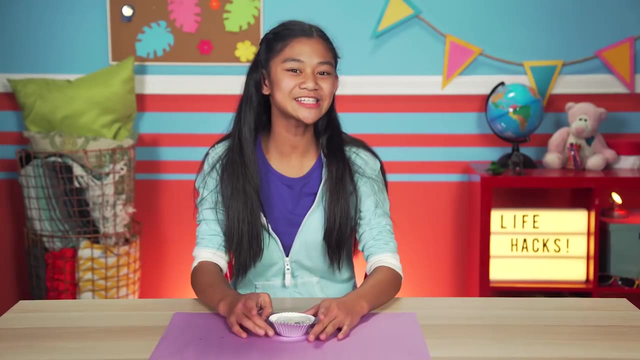 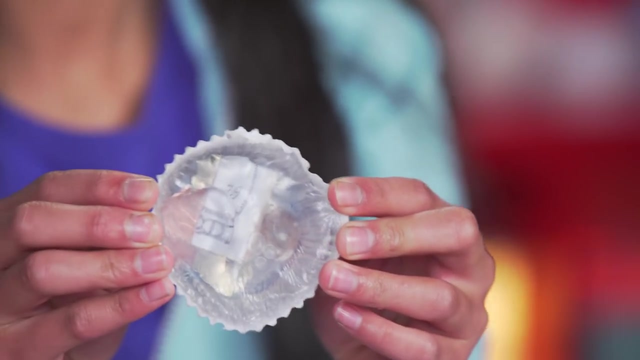 Try to keep the bills and coins in the center of your cupcake foil. Now let it harden for about an hour. Once the soap has hardened, pop it out of your cupcake foil to reveal your money soap. Now, if you give this as a gift, your friends will not only get clean. 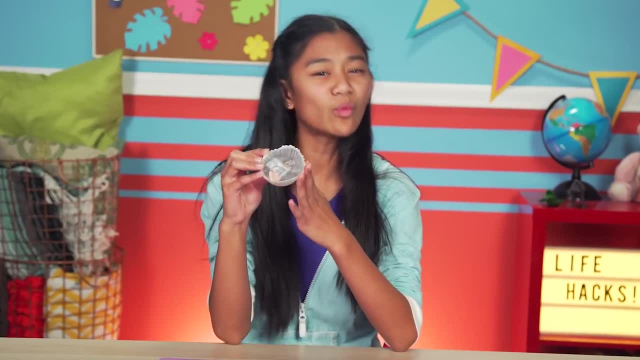 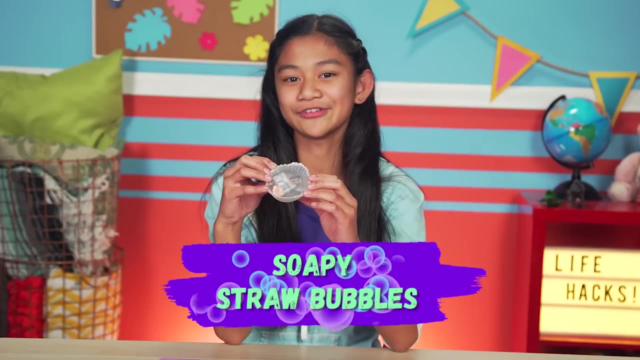 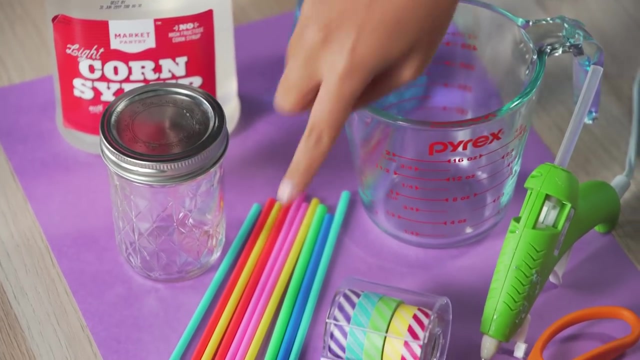 they'll also get rich. And now, if you want to give a gift that will ensure your friends are covered in suds, my next hack is perfect. Here's how to make my soapy straw bubbles. For this hack, you'll need corn syrup, dish soap, a small jar, a measuring cup, straws, washi tape, a glue gun, scissors and a spoon. 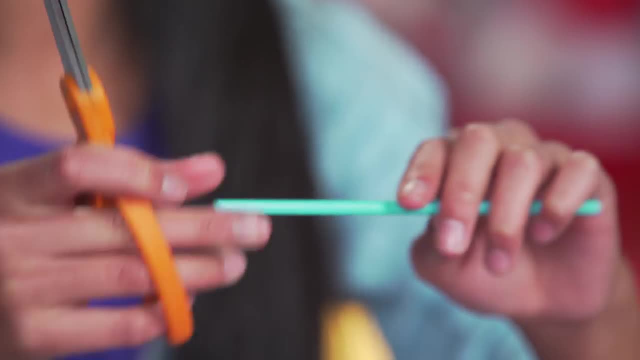 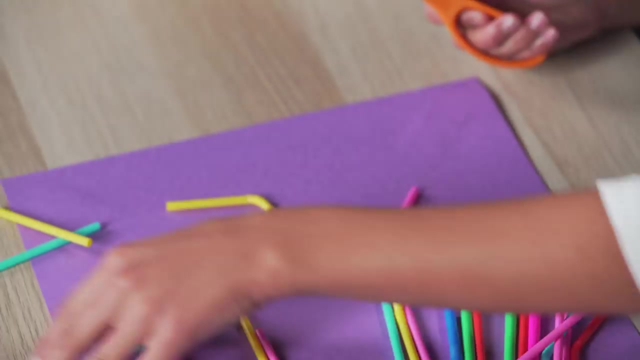 First cut the bendy part of the straw off and then the remainder in half. Cut as many straws as you want, And remember the more straws, the bigger the bubble blower. Glue one straw to the other. Be careful when you're working with hot glue. 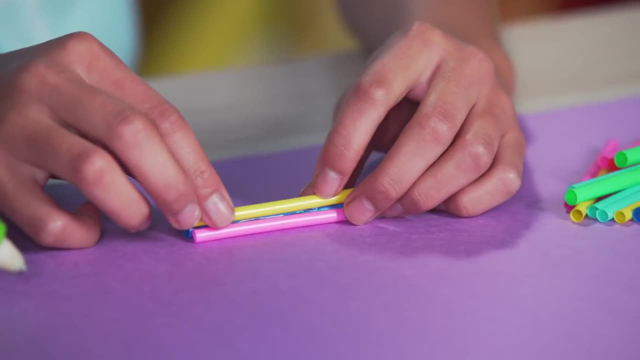 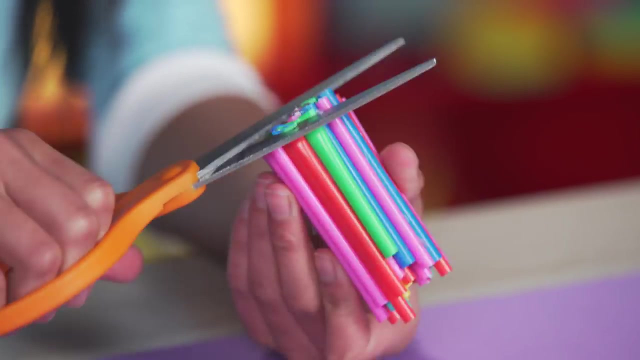 Now glue the next straw to the first two. Keep adding straws until you have the bubble blower you want. Now this isn't quite even. Let's trim it. Trimming this will make sure that the bubbles get on all the straws. 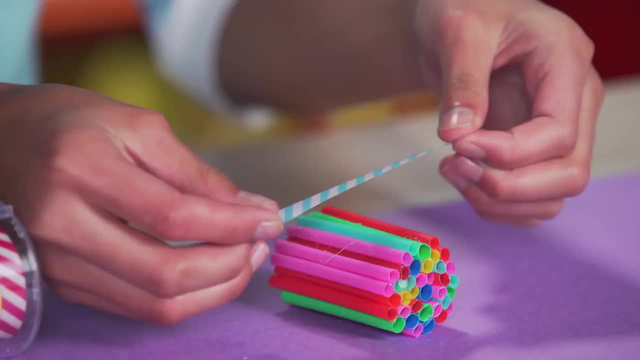 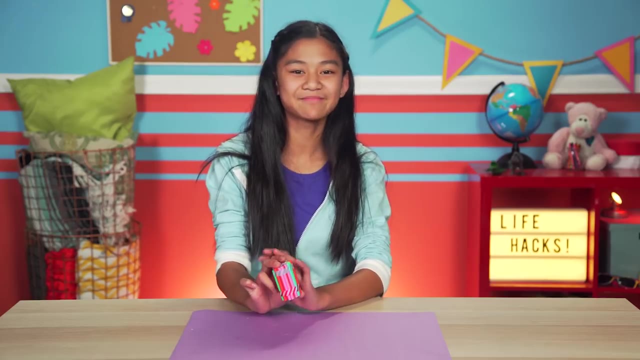 It's like confetti. Yay. Now use some washi tape to decorate your bubble blower. Now that my bubble blower is made, I just need one thing: My bubble solution. Pour one and a half cups of water into your measuring cup and then add a quarter cup of dish soap.